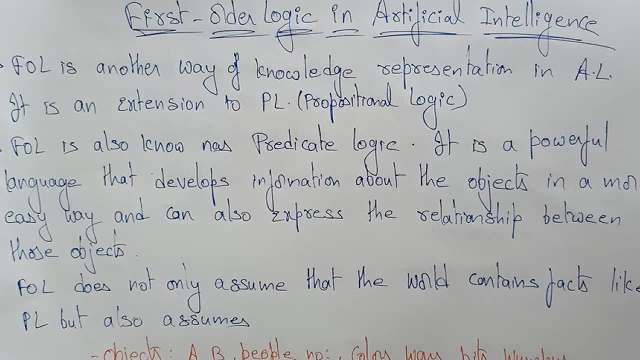 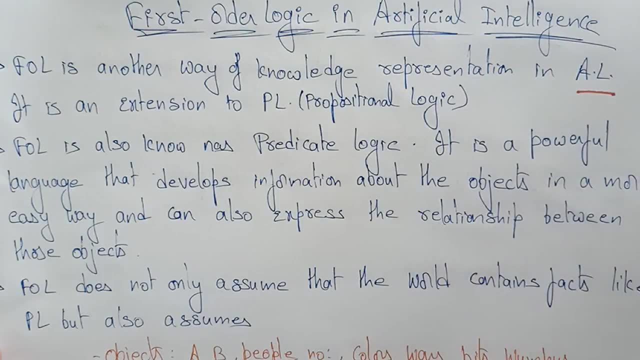 FOL, The first order logic. So let's see, The first order logic is another way of knowledge representation in Artificial Intelligence. So it is in just an extension of the prepositional logic. So if you want to know about this prepositional logic, just go through my videos. 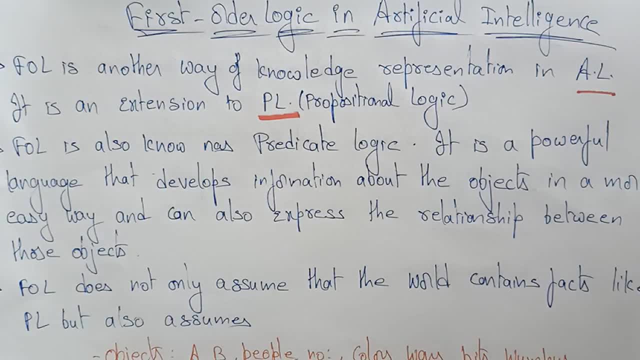 So after that, come to this first order logic, because it's just an extension of that PL, The prepositional logic. Whatever the features that the prepositional logic is having combined with the, this first order logic is implemented. So the main use of the 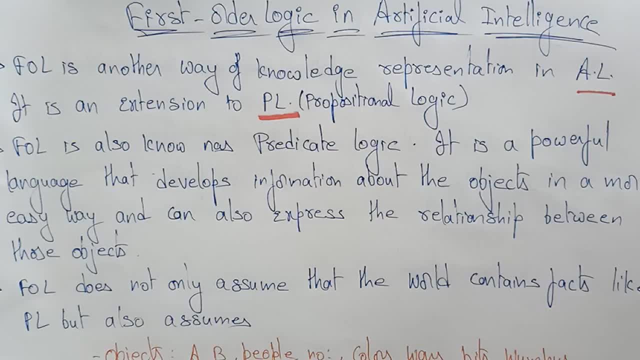 first order logic is to represent the way means. it's just a way of knowledge. It is representing. in Artificial Intelligence It is also called as a predicate logic. The first order logic is also known as first order predicate logic. It is a powerful language. 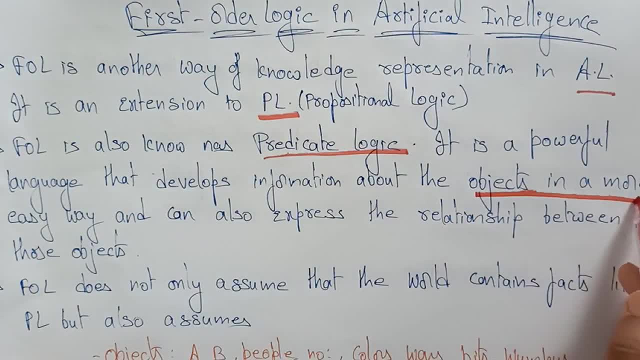 that develops information About the objects in a more easy way and can also express the relationship between those objects. So here the concept is, whereas in the prepositional logic it's only talks about the facts. Either it can. the statement is true or false. But here not only that, the first order logic is develops the 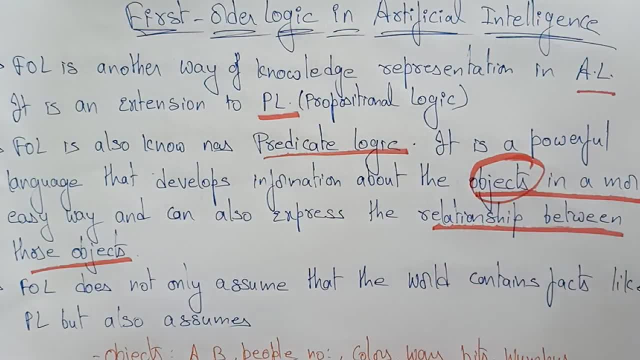 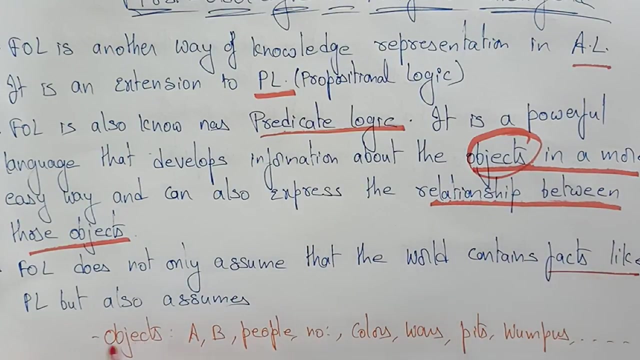 information about the objects, Not only the objects and the relationship between those objects. That everything will be explained in the first order logic Means that the knowledge is presented in the form of objects and the relationship between those objects, and it explains about the facts also. So the first order logic does not only assumes that the world contains the facts, like 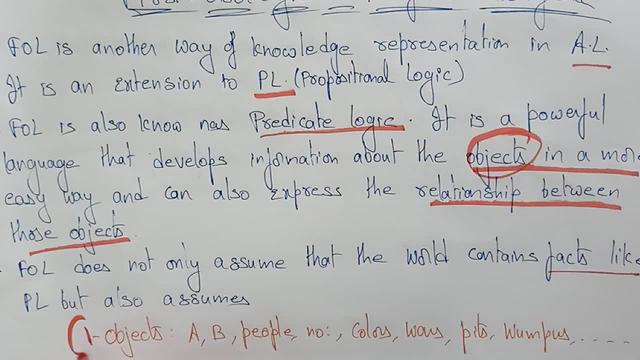 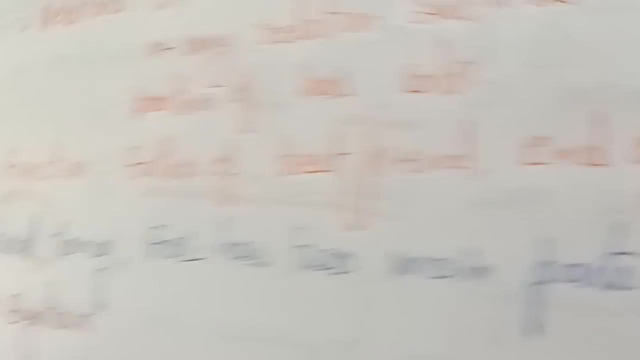 prepositional logic, but also assumes one thing: objects. okay. So not only the facts. the facts is one thing and it also assumes the objects. Objects are nothing but the terms, like a, b, people, some colors, numbers, Whatever it means, pits, whampers, those are. all comes under the objects. and next, relationships. 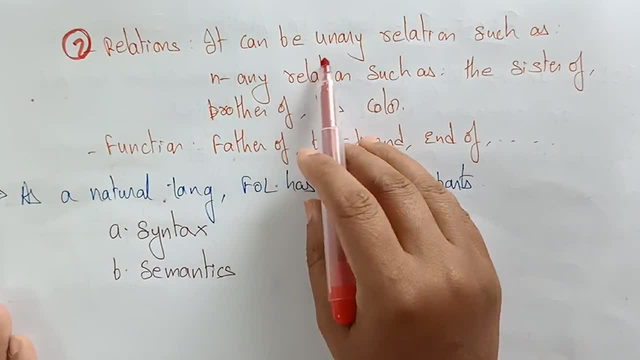 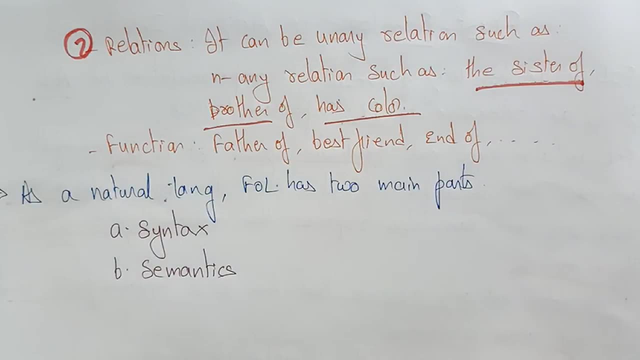 relationships among those objects. It can be unary, relationships such as: and any relations such as the sister of or brother of has color. okay. It not only explains the relationship between the two people, but also it explains the relationship between the unary. it can be represented unary. 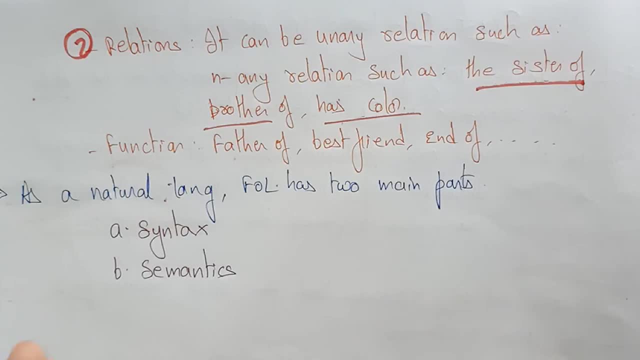 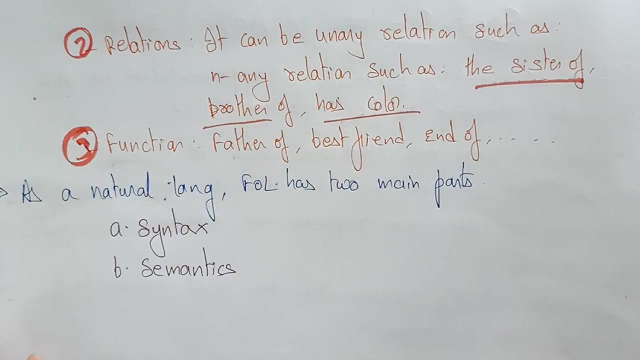 relationships. Let like, uh, she is sister of her- okay, she is. he is the brother of his, like this. and it has a beautiful, uh, that red color like that. okay, it just explains the relationship between those objects. and the third thing is the functions. the father of best friend and off. so this is the functions. so the first order, logic. 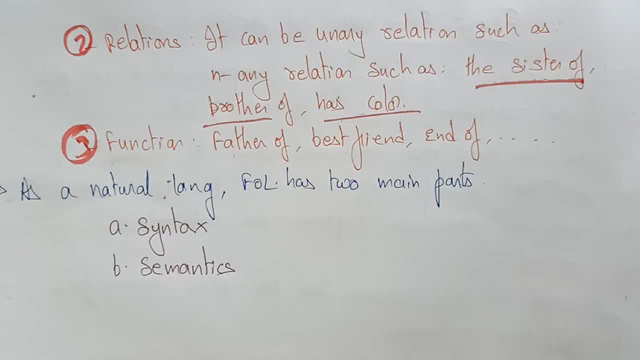 is not only deals with the facts, it also deals with the objects, relationships and the functions. okay, so as a natural Language, the first order logic has mainly two parts. one is the syntax and semantics. so in the preposition logic also, it that uh, the statement can be represented as in: i mean, it can be uh, the. 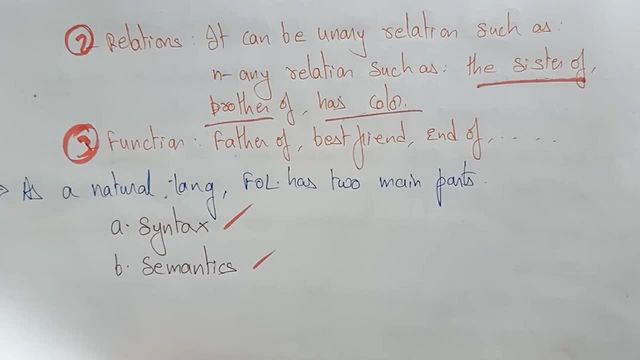 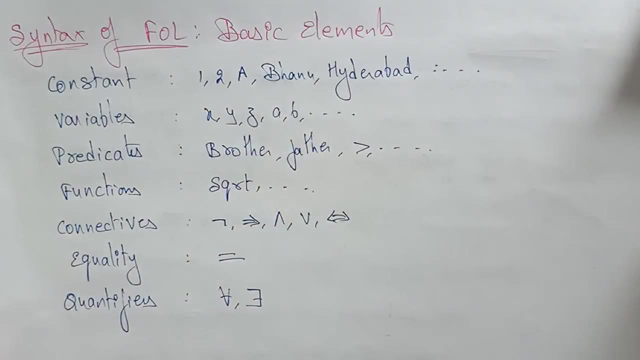 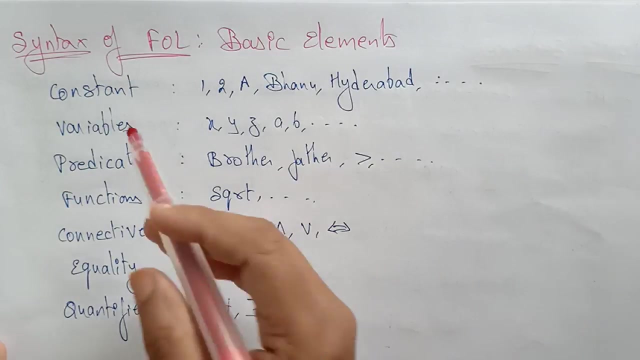 preposition logic also having the two parts. one is the syntax and semantics. in here also, the first order logic has the two main parts: syntax and semantics. now let's see the syntax of first order logic basic elements. so what are the main basic elements here? The basic elements of these? uh, first order logic is constants, variables, predicates, functions. 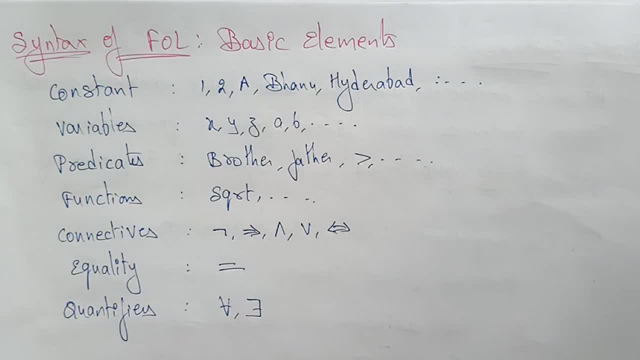 connectivities, equalities and quantifiers. by using all these syntax terms. uh, with the help of these syntax terms, we are going to represent the knowledge of first order logic in artificial intelligence. okay, so the constants, or we call it as the numbers and alphabets, and some names or all. 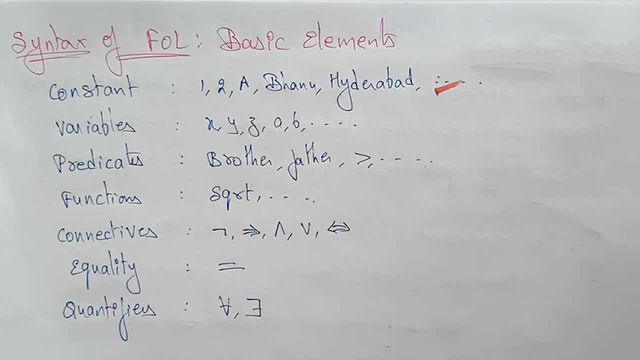 comes under the constant Means they are only uh, work for that particular thing. it's just a constant. and the variables means you can change. instead of these variables you can substitute the another variable also. okay, these are all the variables and predicates. the predicates are: the brother of the father of 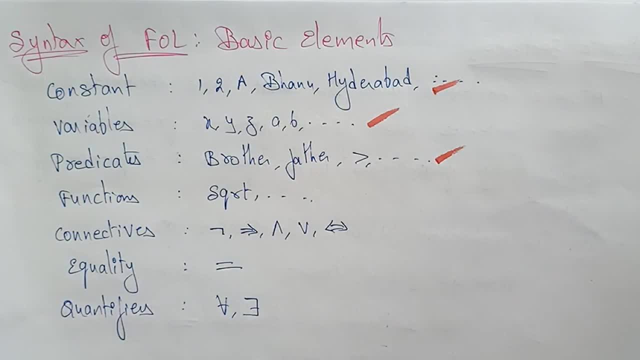 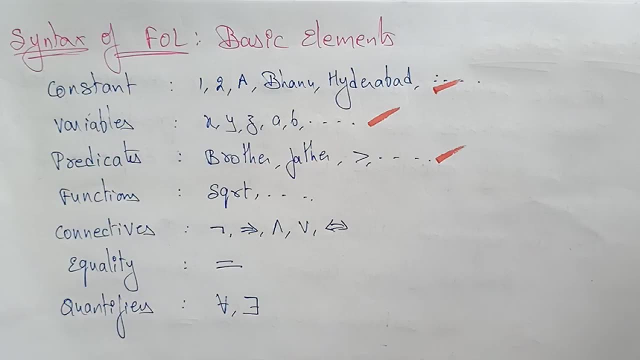 as greater than or equal to so. like that means, uh, greater than less than so. those are comes under the predicates and the functions are the. what type of operation it is going to perform. that is a square root like that. and the collectivities these are used to represent, the. whatever the relationship between those.